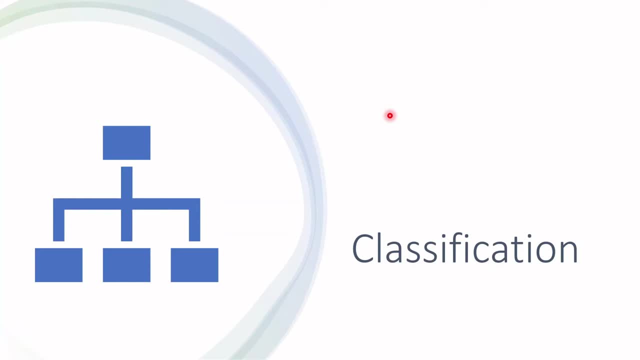 scramble together one with another, and well, hopefully this video will help you make sense of everything. Now, suppose we want to train some sort of classification model that will help us predict whether someone has a certain disease or does not. If someone has a disease and we refer. 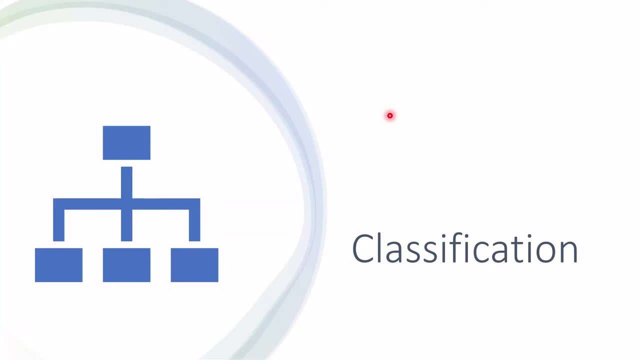 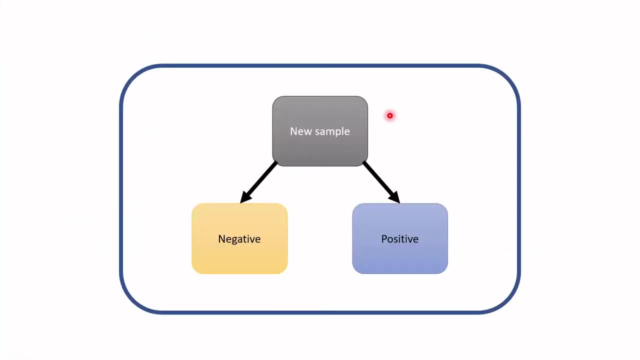 to that as a positive sample. and if someone doesn't have the disease, then we refer to that as a negative sample. And when we have this classification model and a new person, a new sample arrives, then that model is going to help us make sense of everything. So let's get started. 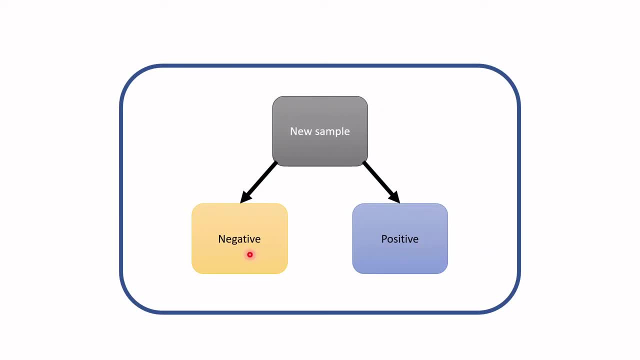 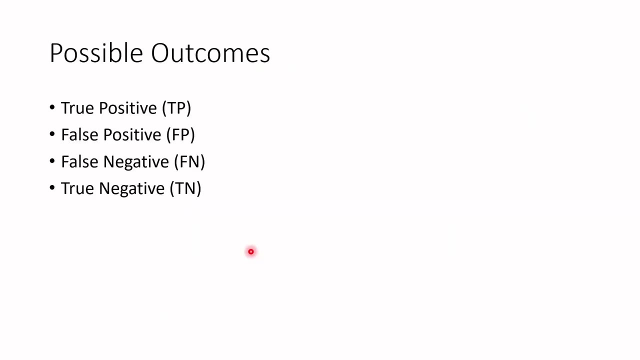 The classification model should be able to predict whether it's a positive or negative sample, And when we look at the outcome of the model compared to the real world, we can divide these outcomes into four different groups: True positive, false positive, false negative and true- negative. Now 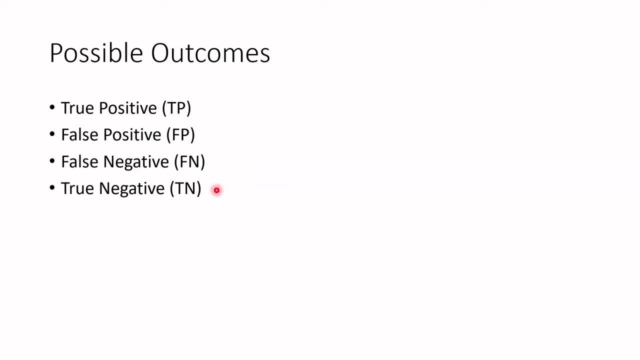 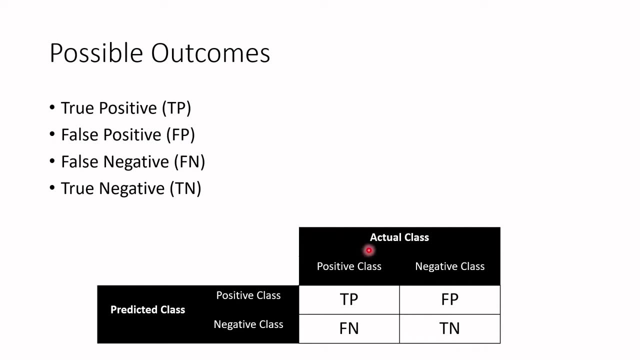 to kind of understand these definitions better, let's use this table down here below, which is also referred to as a confusion matrix. Now, if we only look at the actual class and the positive class, well, everyone who has the disease, if the model was correct and predicted. 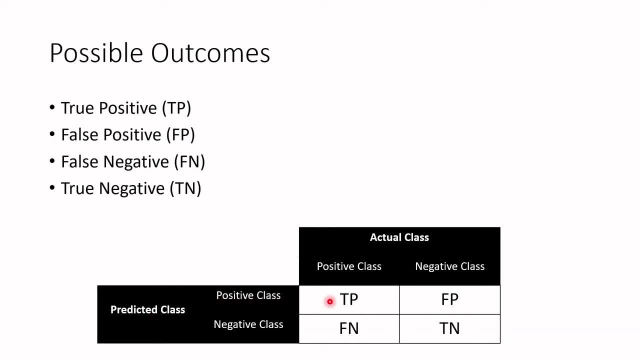 some instance someone as positive, then we refer to that as a true positive sample. So, looking at the positive class, if the model was incorrect, we refer to that as a falsely predicted negative. Again now, looking only at the negative class if the model was incorrect. 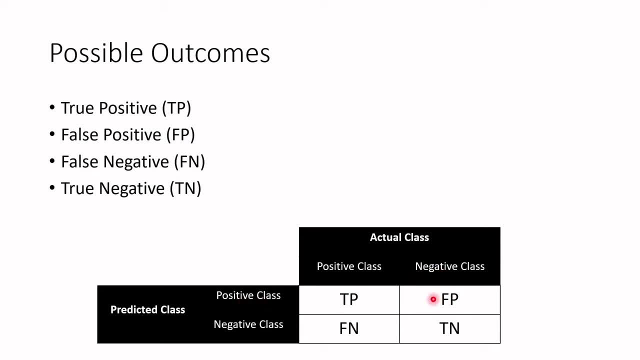 and predicted it as positive, then we refer to that as a false positive. And if the model was correct and predicted it as negative, then we refer to that as a true negative. Okay, now there's a few other notes I would like to say regarding this slide. One is: well, it's easy. I guess it would be easiest. 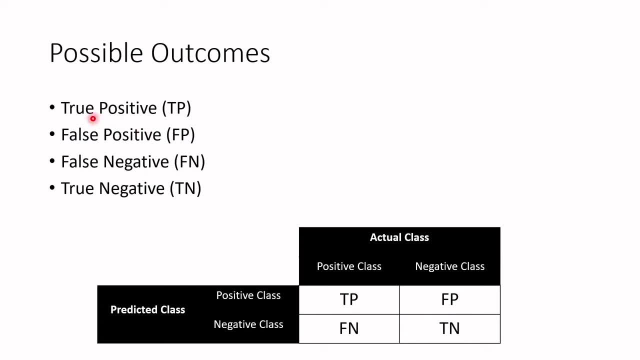 to remember what's everything If you remember that everything that's true, well, the model was correct about, And everything that is false, the model was incorrect about. Regarding the false positive, it is also referred to as well, sometimes as type one error. 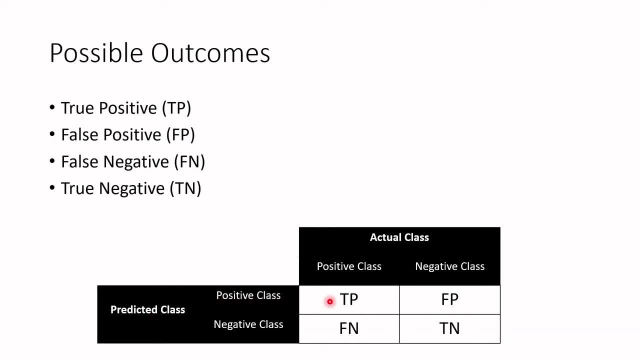 some instance someone as positive, then we refer to that as a true positive sample. So, looking at the positive class, if the model was incorrect, we refer to that as a falsely predicted negative. Again now, looking only at the negative class if the model was incorrect. 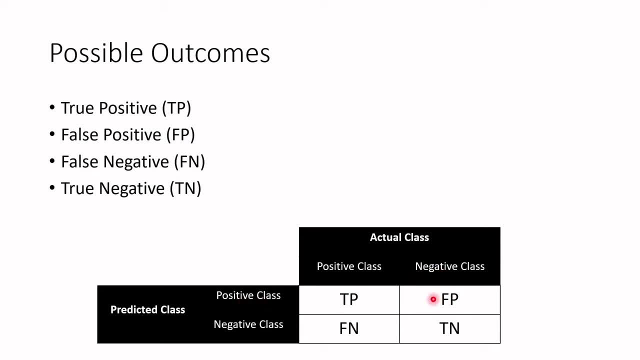 and predicted it as positive, then we refer to that as a false positive. And if the model was correct and predicted it as negative, then we refer to that as a true negative. Okay, now there's a few other notes I would like to say regarding this slide. One is: well, it's easy. I guess it would be easiest. 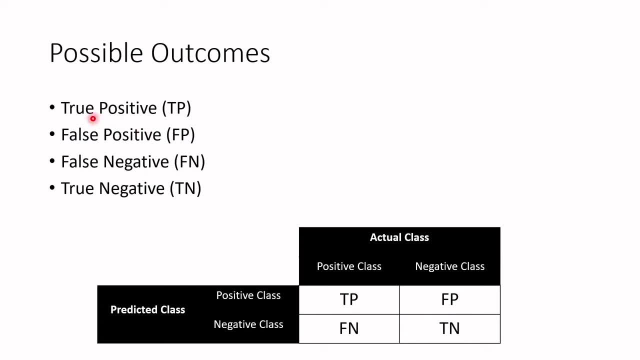 to remember what's everything If you remember that everything that's true, well, the model was correct about, And everything that is false, the model was incorrect about. Regarding the false positive, it is also referred to as well, sometimes as type one error. 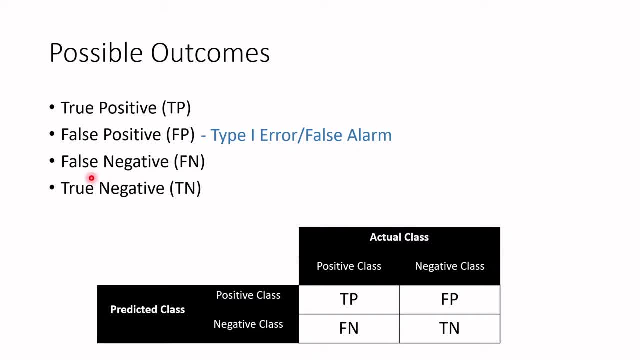 And sometimes as a false alarm- And the false negative is sometimes referred to as well- a type two error. Another thing you might want to notice is that, well, if you look at other tutorials and other videos which explain this, then sometimes people switch. 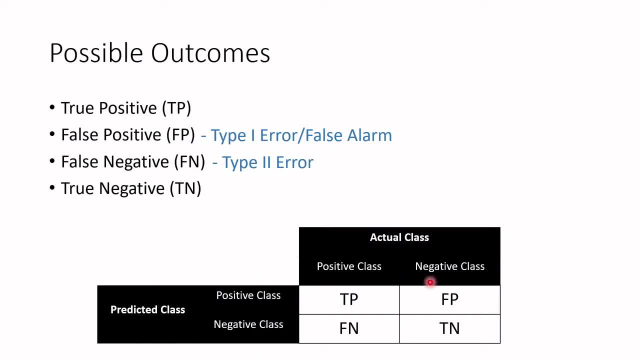 the actual class and the predicted class, And that results in the definitions inside also changing places. So you want, you might want, to pay attention to that as well. Now, moving forward, what we want to do is to understand these definitions better through. 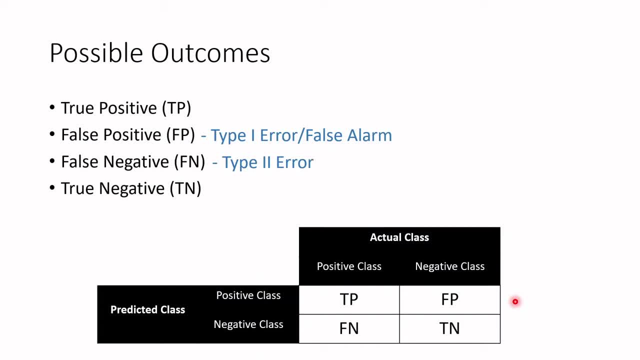 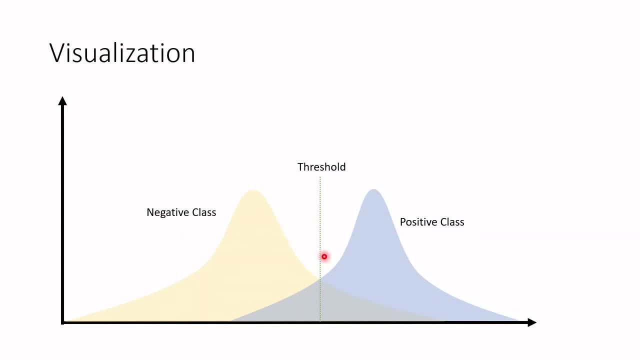 visualization. So we'll take a look at two different visualizations. In the first one, what we have is, well, the two different distribution- The positive people who have the disease, and the negative people who do not have the disease, And the horizontal axis over here can. 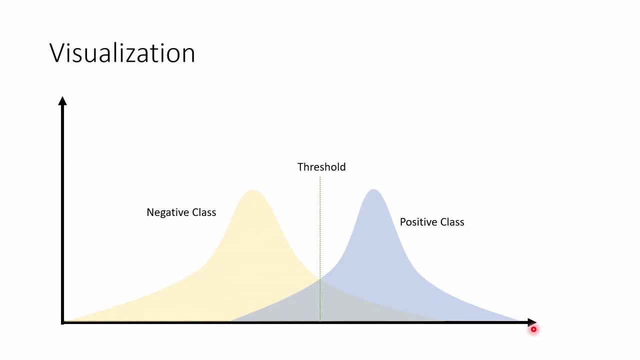 represent well, whatever we want. I mean, oh, if we're talking about a disease, maybe a good idea to represent it as well. maybe some sort of medical test that has a numerical value, Maybe a blood test with a numerical value. And the y-axis, the vertical axis, represents. 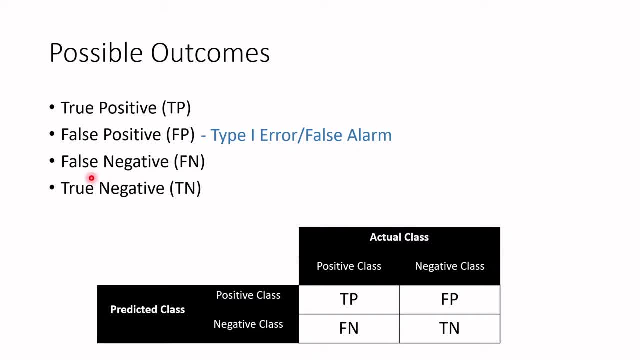 And sometimes as a false alarm- And the false negative is sometimes referred to as well- a type two error. Another thing you might want to notice is that, well, if you look at other tutorials and other videos which explain this, then sometimes people switch. 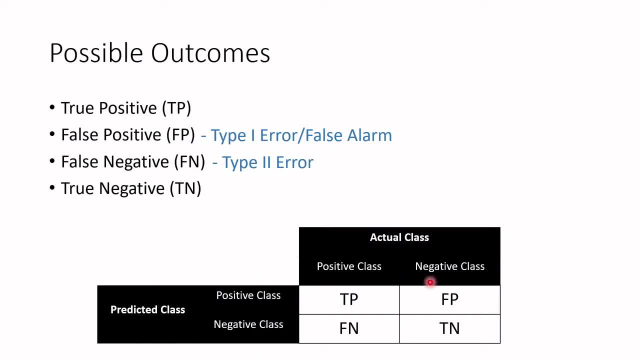 the actual class and the predicted class, And that results in the definitions inside also changing places. So you want, you might want, to pay attention to that as well. Now, moving forward, what we want to do is to understand these definitions better through. 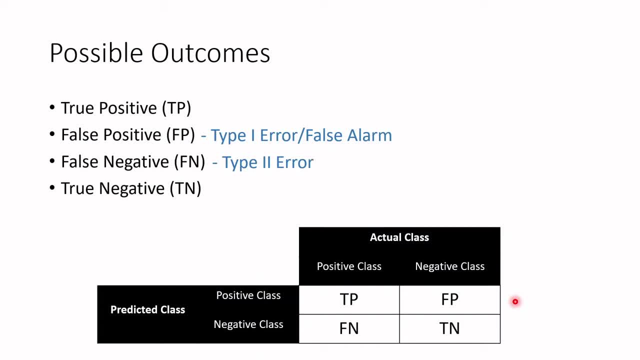 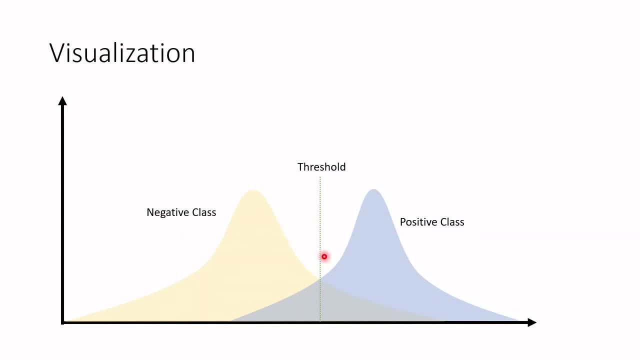 visualization. So we'll take a look at two different visualizations. In the first one, what we have is, well, the two different distribution- the positive people who have the disease, and the negative people who do not have the disease, And the horizontal axis over here can. 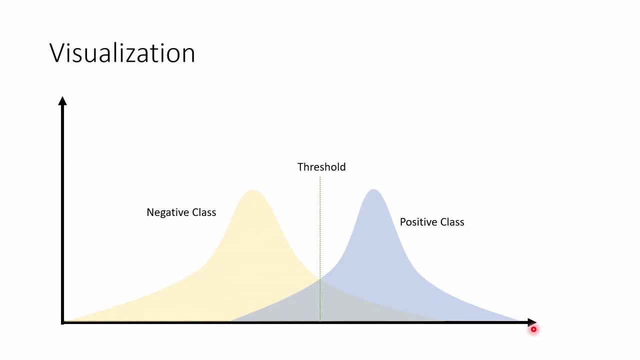 represent well, whatever we want. I mean, oh, if we're talking about a disease, maybe a good idea to represent it as well. maybe some sort of medical test that has a numerical value, Maybe a blood test with a numerical value. And the y-axis, the vertical axis, represents. 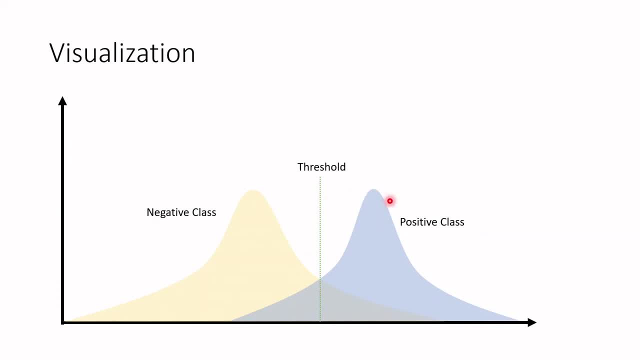 the number of people, the number of samples. So, looking only at the positive class, well, relatively, there are many people in the positive class who have these values of the medical test value. And well, when we train a model, we get a threshold, And then when a new instance arrives, 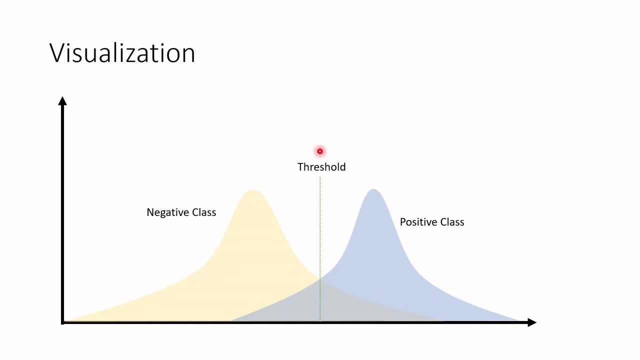 and on that new instance- we do not know if it has or does not have the disease- and that instance takes the medical test. if the value is above the threshold, then the model would predict it as a positive sample, And if it's below, then the model would predict it as: 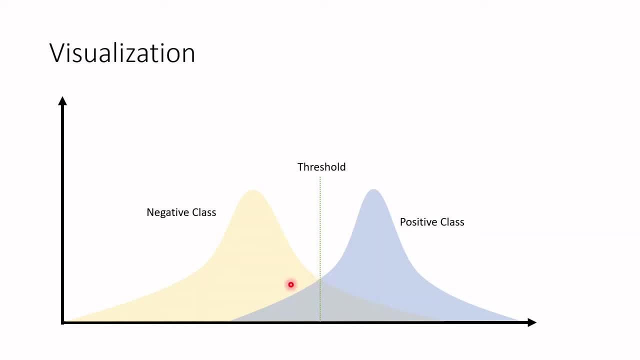 a negative sample And you can see by this visualization that the threshold divides our data into four different groups, Connecting that to the previous slide. again, looking only at the positive class, the threshold divides it into the truly predicted positive and the falsely predicted negative. 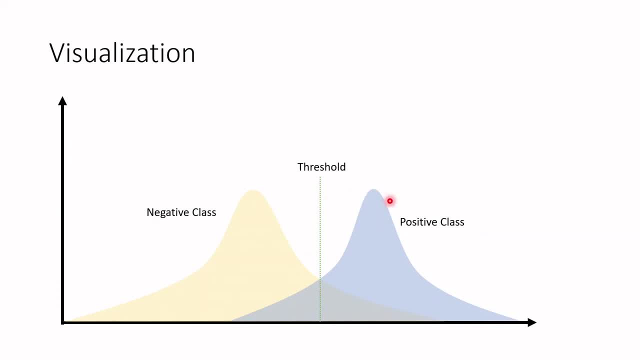 the number of people, the number of samples. So, looking only at the positive class, well, relatively, there are many people in the positive class who have these values of the medical test value. And well, when we train a model, we get a threshold, And then when a new instance arrives, 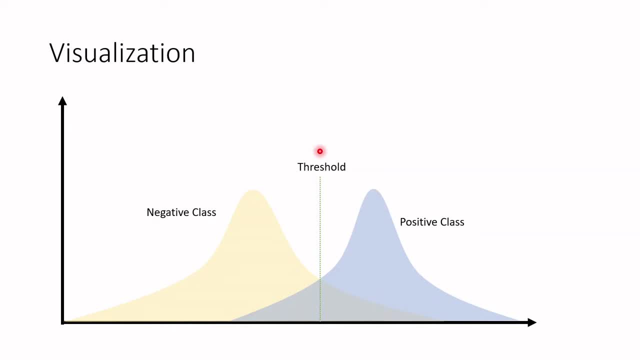 and on that new instance- we do not know if it has or does not have the disease- And that instance takes the medical test. If the value is above the threshold, then the model would predict it as a positive sample, And if it's below, then the model would predict it as a negative sample. 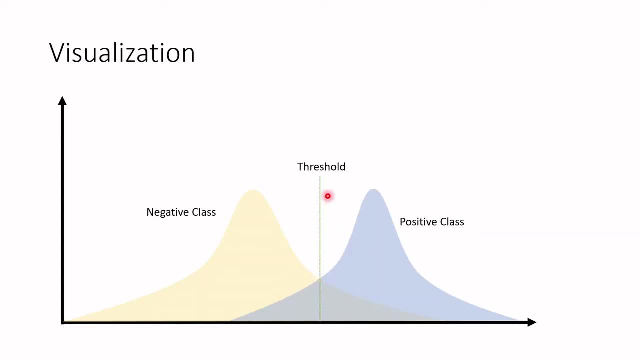 And you can see by this visualization that the threshold divides our data into four different groups, Connecting that to the previous slide. again, looking only at the positive class, the threshold divides it into the truly predicted positive and the falsely predicted negative. And looking 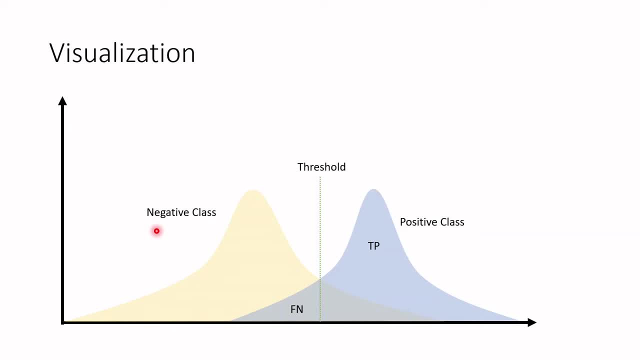 only at the negative class. the threshold divides it into the truly predicted negative and the falsely predicted positive. Let's move forward to talk about the next visualization. Over here we have the two different classes, And our model prediction is represented by this blue. 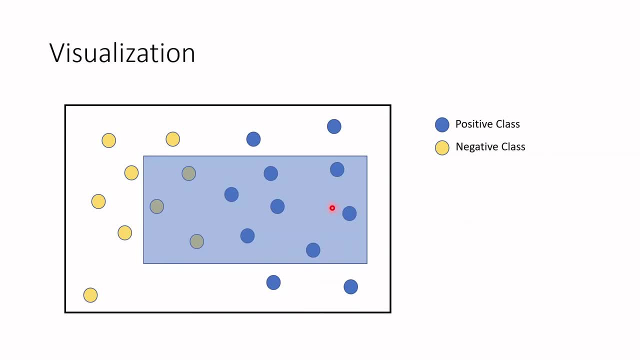 rectangle over here. So anything inside this blue rectangle over here our model predicts as positive And we connect that again to what we saw in the previous slide. So looking only at the positive class, we can divide it into two different groups: the truly predicted, positive and well. 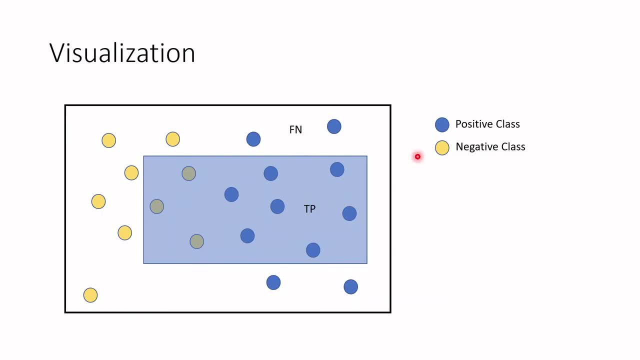 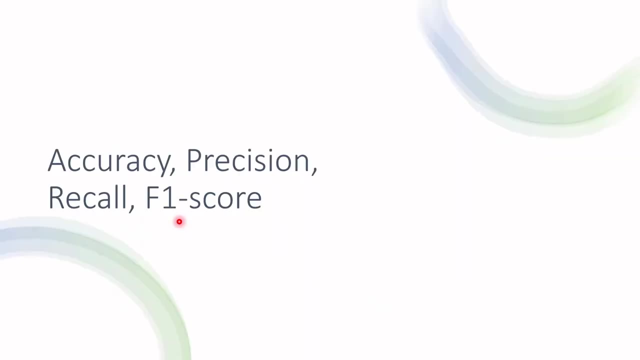 whatever is outside and is the falsely predicted negative. And looking only at the negative class, it's again divided into two groups: the truly predicted negative and the falsely predicted positive. Okay, Next we are going to talk about, well, these definitions which are widely used in machine. 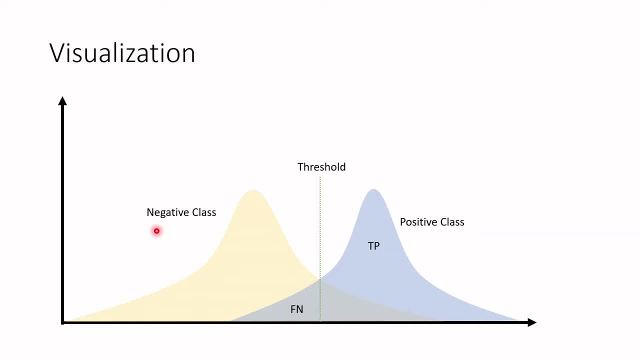 And looking only at the negative class, the threshold divides it into the truly predicted negative and the falsely predicted positive. Let's move forward to talk about the next visualization. Over here we have the two different classes, and our model prediction is represented by 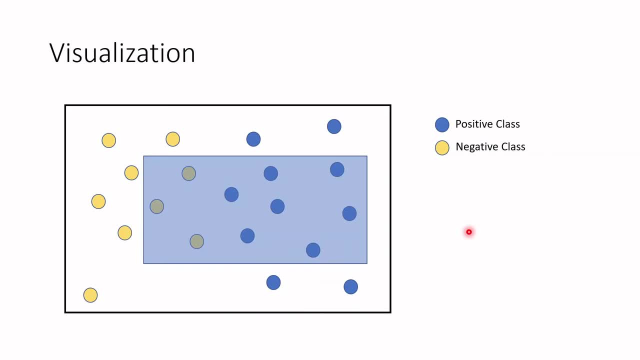 this blue rectangle over here. So anything inside this blue rectangle over here our model predicts as positive And we connect that again to what we saw in the previous slide. So, looking only at the positive class, we can divide it into two different groups: the 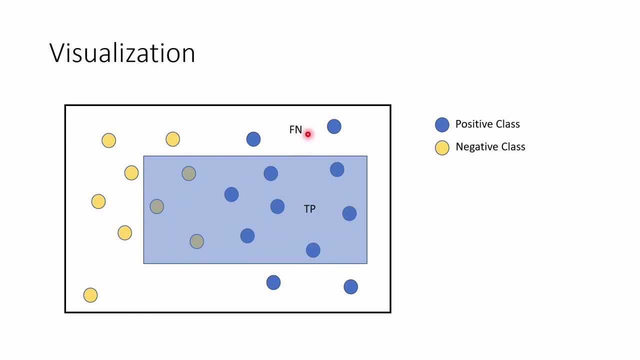 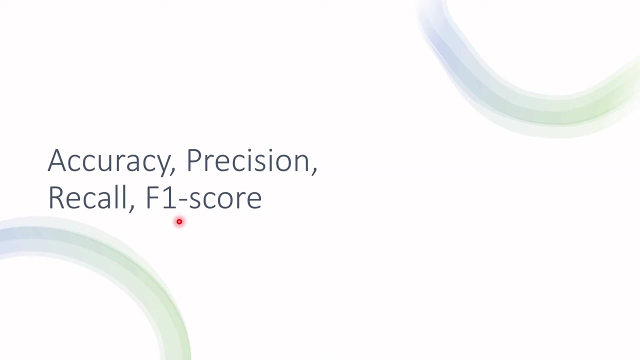 truly predicted positive. and well, whatever is outside, And it's the falsely predicted negative, And looking only at the negative class, it's again divided into two groups: the truly predicted negative and the falsely predicted positive. Okay, Next we are going to talk about: well, these definitions which are widely used in machine. 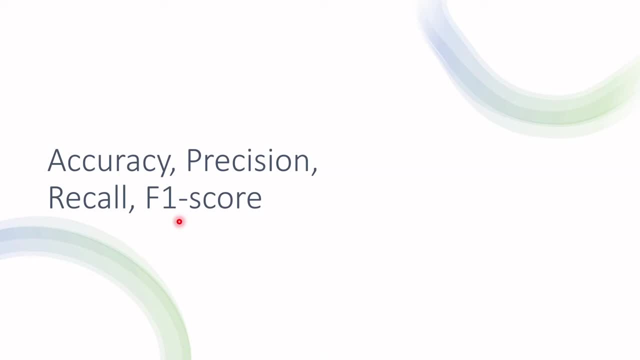 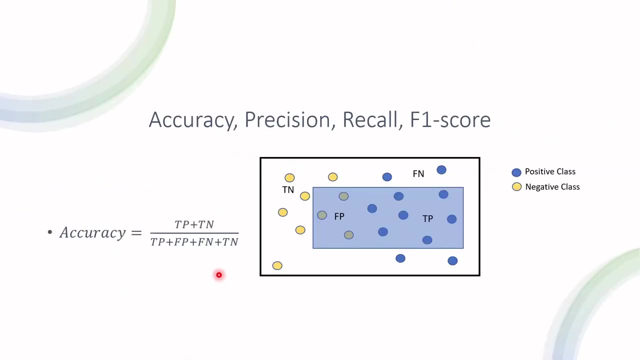 learning and data science and statistical analysis, And it's very important to understand what they mean. Let's start with accuracy, which I guess it's easiest to understand and probably also easiest to explain as well. Accuracy is defined as whatever is true or truly predicted, true positives and true negative. 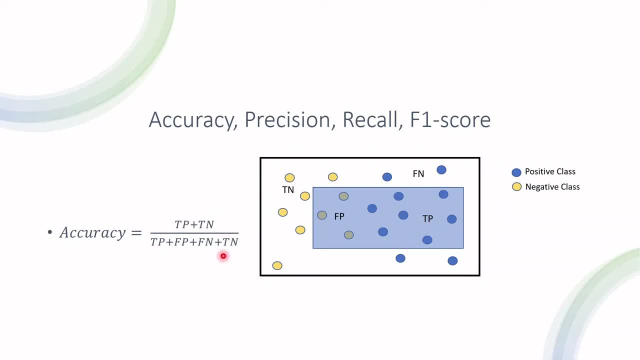 divided by well everything. So, if I'd had to put it in words- is well. how well did your model perform regarding the two different classes, positive and negative? How many instances was the model correct about Moving forward? let's talk about precision. 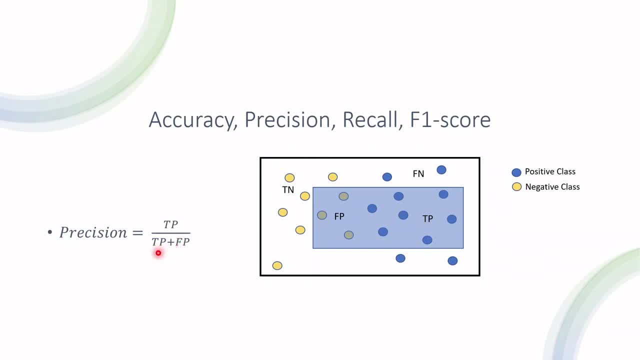 Precision is defined as true positive, divided by true positives and the false positives. Well, whatever is inside this blue rectangle, So trying to put that into words, it's: how well did your model perform regarding its prediction of the positive class Moving forward? let's talk about recall. 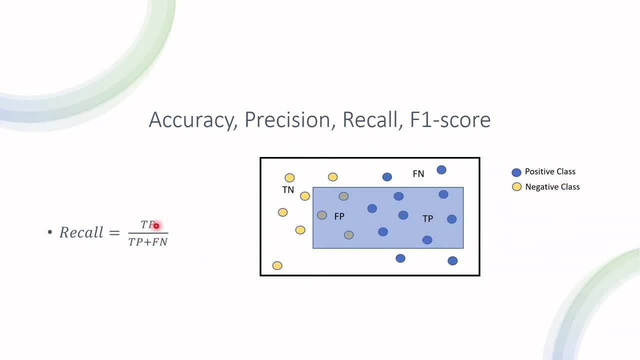 Recall is defined as well: true positive, divided by true positive and the false negative. So well again, trying to put that into words. recall is defined as well out of the positive class. how well did your model perform? 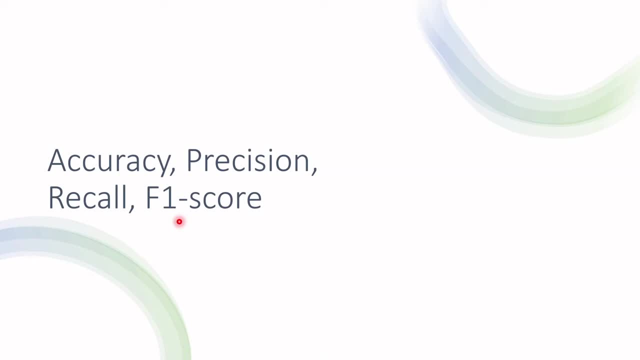 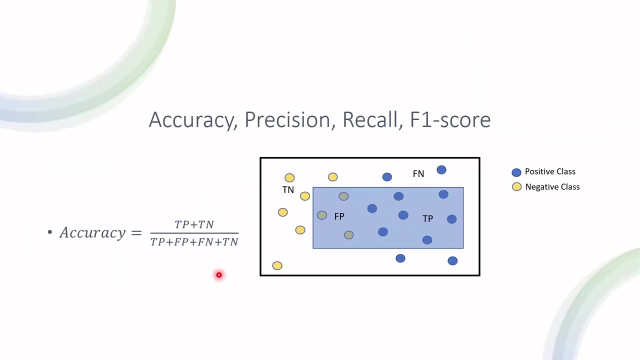 learning and data science and statistical analysis, And it's very important to understand what they mean. Let's start with accuracy, which I guess it's easiest to understand and probably also easiest to explain as well. Accuracy is defined as whatever is true or truly predicted true positives. 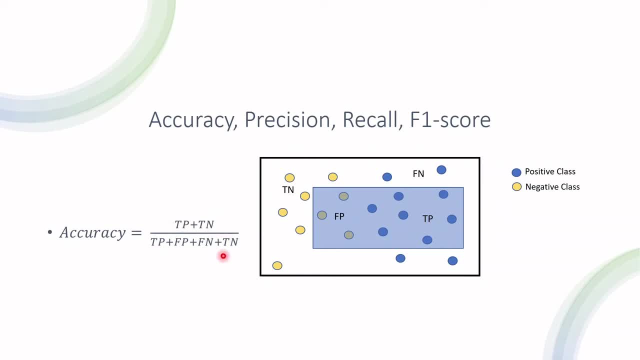 and true negatives divided by well everything. So if I had to put it in words, it's: how well did your model perform regarding the two different classes, positive and negative? How many instances was the model doing so clearer? How many times did the model do it? 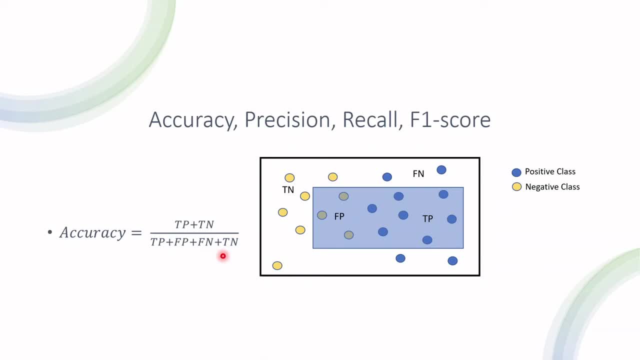 in different ways. How often was the model giving activities? How many times was the model нравитсяing the whole thing? How many instances was the model appreciating something? the model correct about moving forward. let's talk about precision. precision is defined as true positive, divided by true positives and the false positives. well, 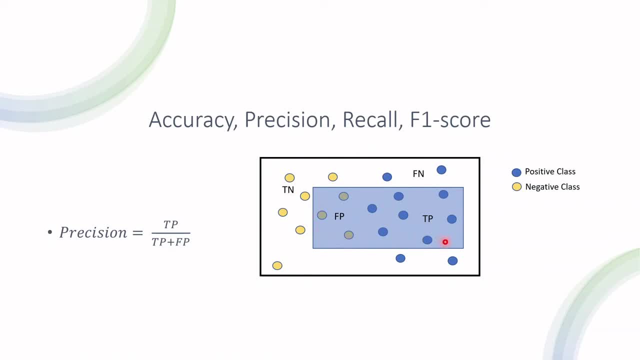 whatever is inside this blue rectangle. so, trying to put that into words, it's: how well did your model perform regarding its prediction of the positive class? moving forward, let's talk about recall. recall is defined as well: true positive divided by true positive and the false negative. so well, again trying. 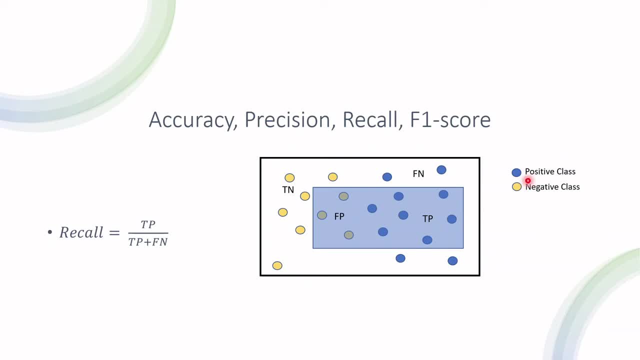 to put that into words, recall is defined as well out of the positive class. how well did your model perform? how many instances were correctly identified as people who have the disease? and the last part in this section is the f1 score which, well, looking at its definition, it's the least intuitive. it's defined as recall times- perfect. 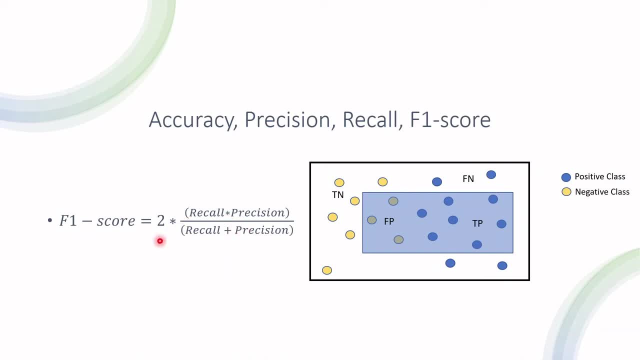 precision divided by recall plus precision, and all that multiplied by 2, which is the harmonic mean of recall and precision, and well, we use f1 score when we compare different models and let's say one model has high precision and the other one has low recall and the other model has high. 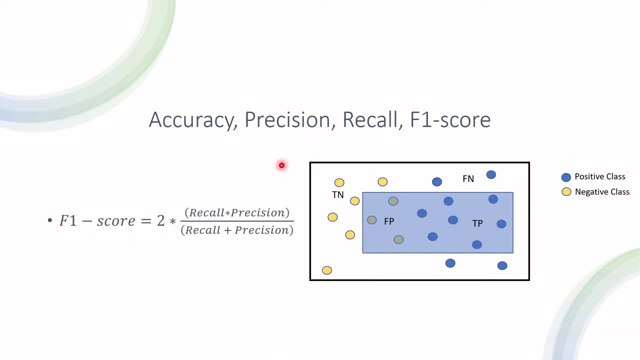 recall and low precision, we really can't tell which one would be better. and well, that's where f1 score comes into the picture. another use for f1 score is that. well, you saw what accuracy does accuracy? well that that calculates how well the model perform regarding the two classes. but if they're not evenly distributed, 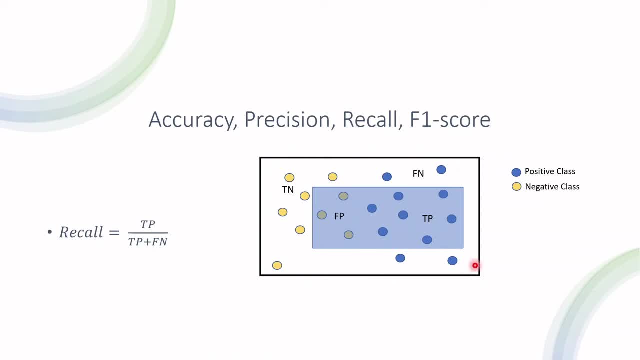 How many instances were correctly identified as people who have the disease. And the last part in this section is the F1 score, Which is the F1 score. It's the F1 score Which, well, looking at its definition, it's the least intuitive. 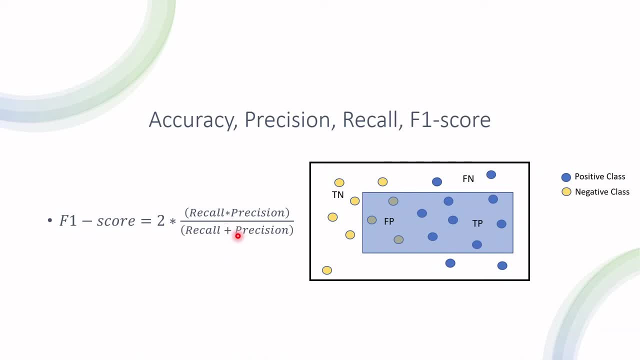 It's defined as recall times, precision divided by recall plus precision, and all that multiplied by two, Which is the harmonic mean of recall and precision. And well, we use F1 score when we compare different models And let's say, one model has high precision and the other one has low recall and the other? 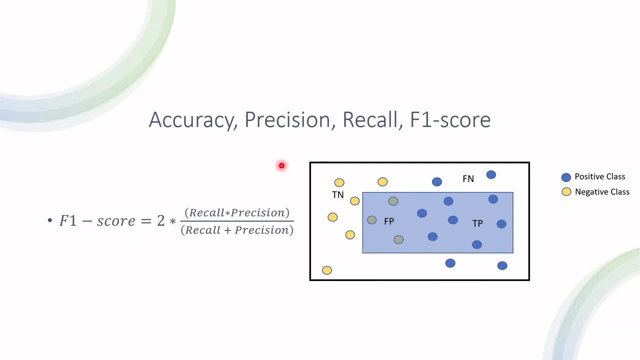 model has high precision And the other model has high precision and the other one has low recall. And if they have high recall and low precision, we really can't tell which one would be better. And well, that's where F1 score comes into the picture. 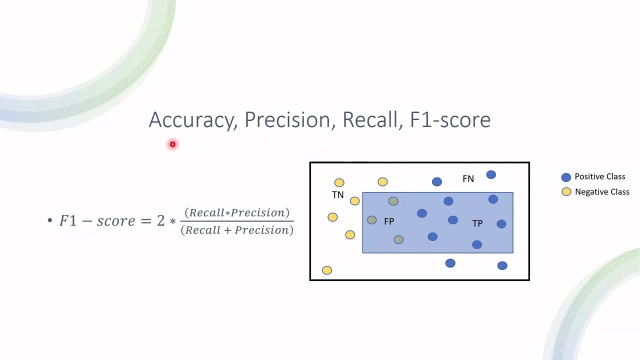 Another use for F1 score is that. well, you saw what accuracy does Accuracy. well, that calculates how well the model performed regarding the two classes. But if they're not evenly distributed, well, then that's where F1 score comes into, the 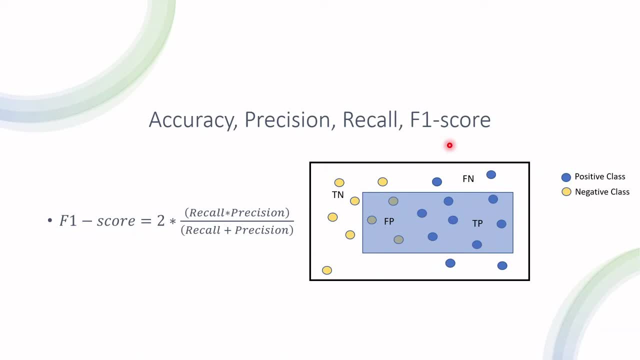 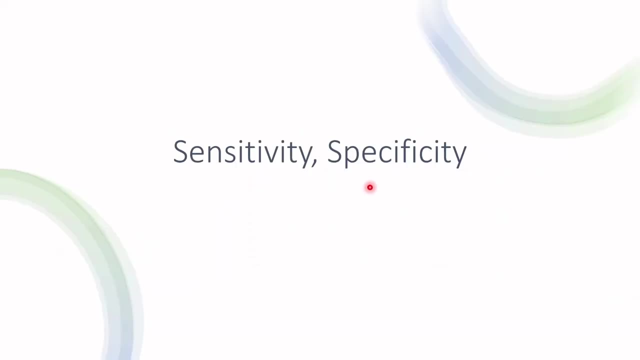 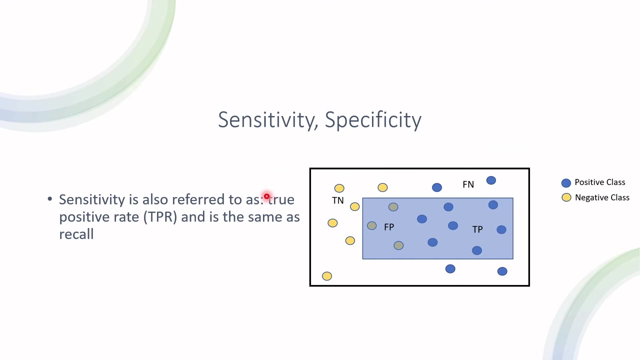 picture and it's a better metric to evaluate the performance of the model. It's also important to know that F1 score is also referred to as F score and F measure. moving forward to our next section, let's talk about sensitivity and specificity. sensitivity has two other names. one is true positive rate and the other is recall. so we 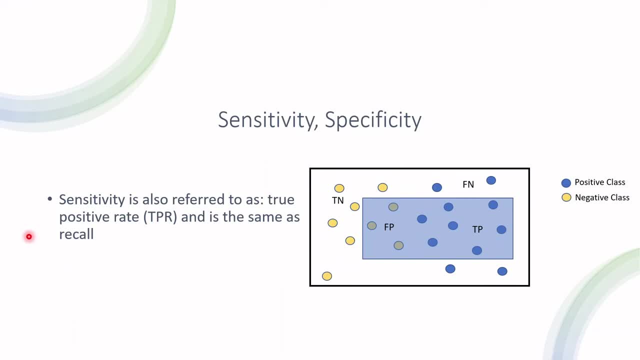 already know what it means. it's the same as recall and it's actually very common in statistical analysis and again, data science and machine learning to for different measures, for the or the same measure to have different names. again, it's very confusing, but it's also important to understand what. what each 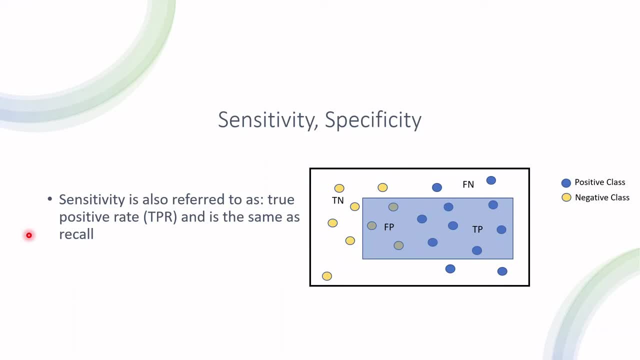 one of these definitions mean. so, if you remember, if you recall, what recall is then sensitivity or recall, or true positive rate? is the true positive divided by true positive and the false negative, which, again putting it in words, is: how well did your model perform? regarding the positive class, specificity is something that we 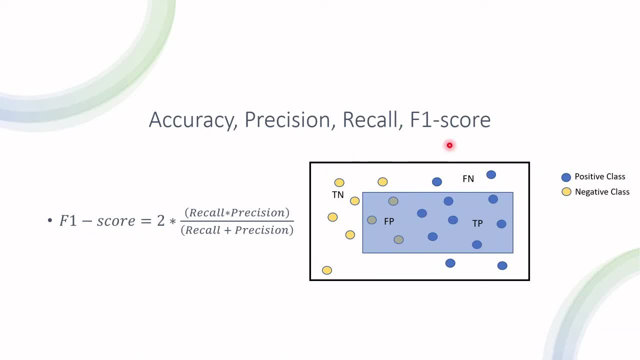 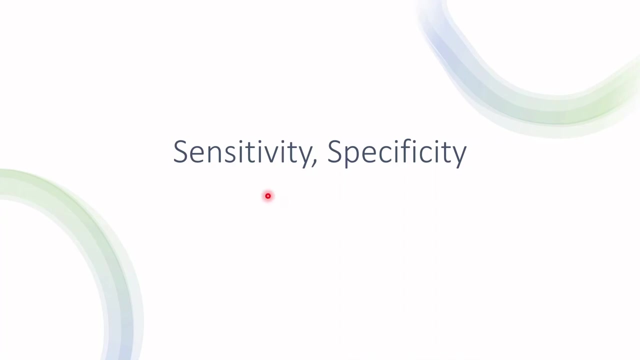 well then, that's where f1 score comes into the picture, and it's a better metric to evaluate the performance of the model. it's also important to know that f1 score is also referred to as f score and f measure. moving forward to our next section, let's talk about sensitivity and specificity. 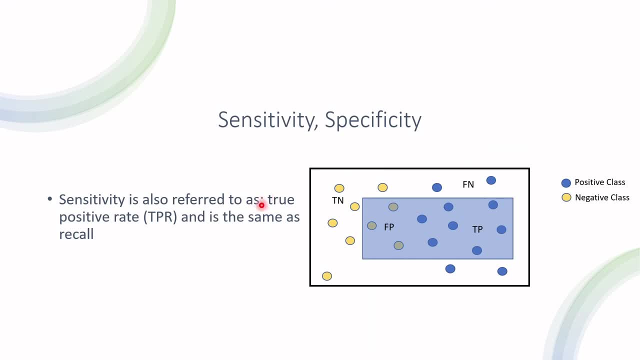 sensitivity has two other names: one is true positive rate and the other is recall. so we already know what it means. it's the same as recall and it's actually very common in statistical analysis and again, data science and machine learning to for different measures, for the, or the same measure to 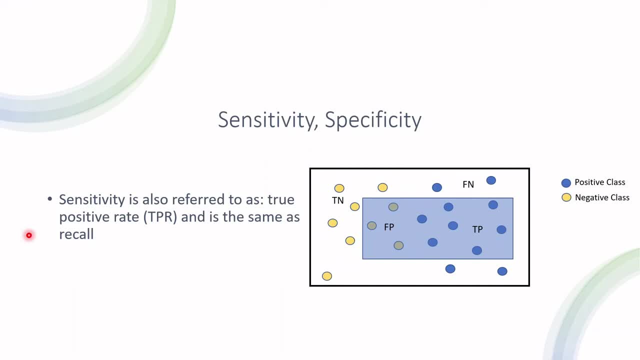 have different names. again, it's very confusing, but it's also important to understand what, what each one of these definitions mean. so, if you remember, if you recall, what we call is then sensitivity, or recall, or true positive rate is the true positive divided by true positives and the false negative. 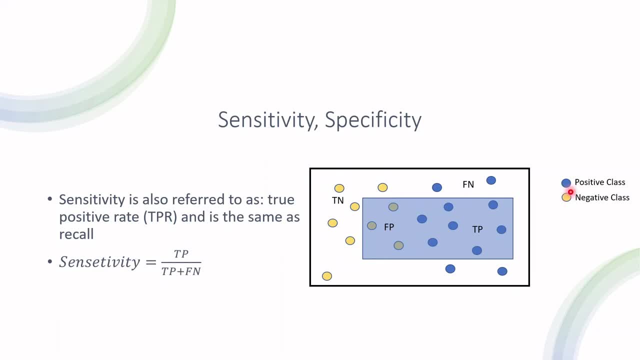 which, again putting it in words, is: how well did your model perform? regarding the positive class, specificity is something that we have not encountered yet and it is referred to, or another name is true negative rate, and it's defined by the true negatives, divided by the true negative and the false positive. 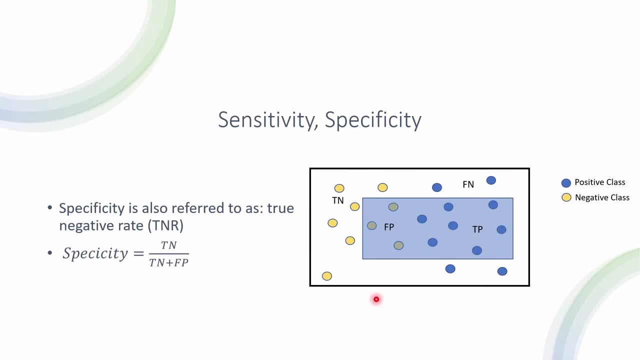 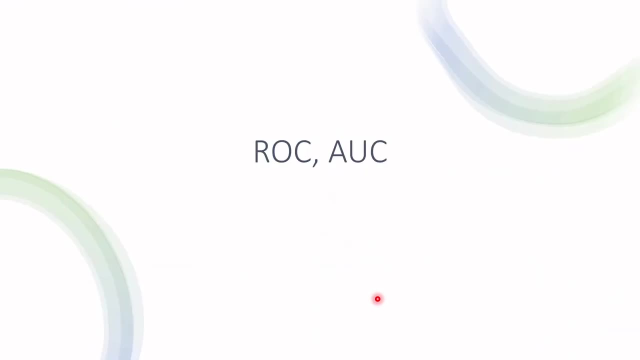 So again, trying to put that into words is: how well did your model perform regarding the negative class? How many instances were correctly identified as negative? Moving forward to our last section, let's talk about ROC and AUC. ROC stands for Receiver Operating Characteristic Curve. 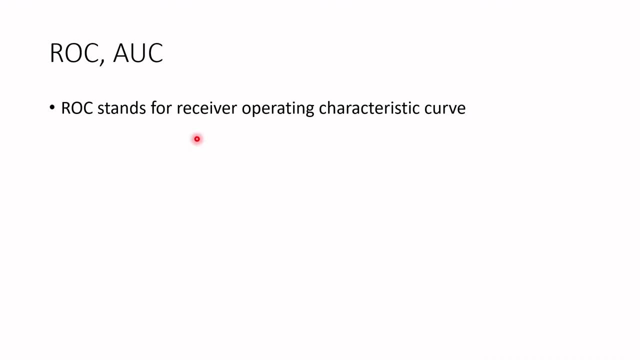 And well, when you hear what something stands for, usually that helps you understand what it means, and I don't think this is the case over here. I will say that ROC was developed somewhere in the 1940s by the military. 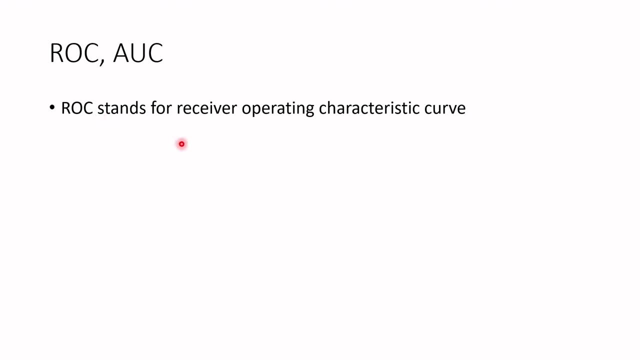 and it was used to evaluate radar systems, and that's where the name comes from. And well, what we do over here is that we calculate for a given model, we calculate for many thresholds. well, that's what we do over here is that we calculate for a given model. 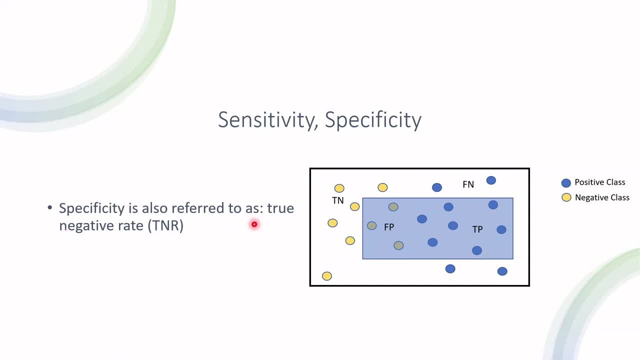 have not encountered yet and it is referred to, or another name is true negative rate and it's defined by the true negatives, divided by the true negative and the false positive. so again, trying to put that into words is: how well did your model perform regarding the negative class? how many instances? 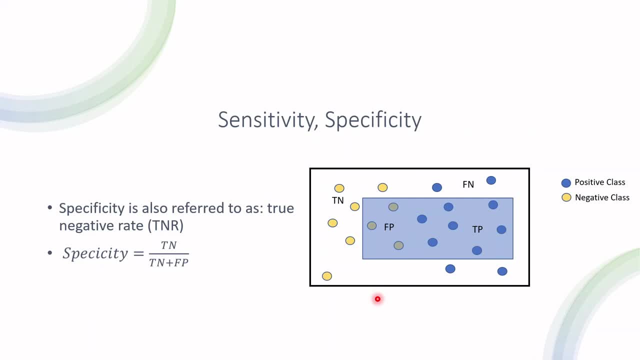 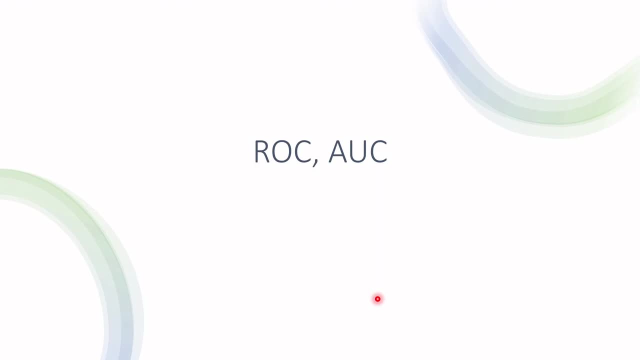 were correctly identified as negative. moving forward to our last section, let's talk about ROC and AUC. ROC stands for receiver operating characteristic, characteristic curve, and well, when you hear what something stands for, usually that helps you understand what it means, and I don't think this is the case over here. I will say that ROC was developed. 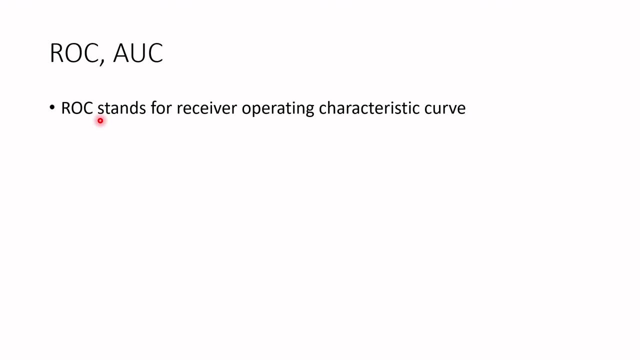 somewhere in the 1940s by the military, and it was used to evaluate radar systems, and that's where the name comes from. and well, what we do over here is that we calculate for a given model. we calculate, for many thresholds, well, the performance of the model, and for each threshold we calculate two different. 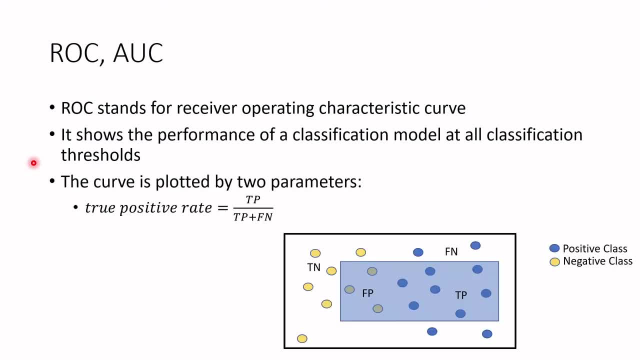 parameters. the first parameter is the true positive rate and, if you remember from the previous slides, it's the exact same thing as recall and sensitivity. it's true positive divided by true positives and the false negative. so how well did your model perform regarding the positive class? the next parameter is: 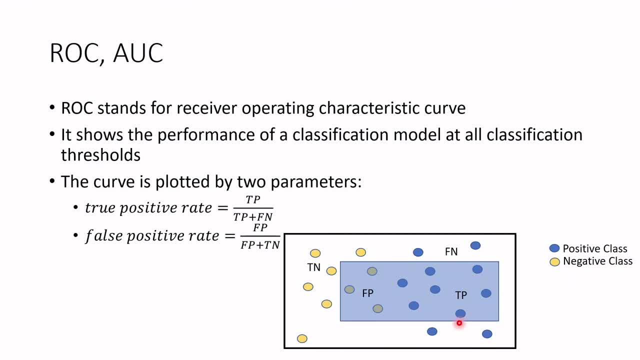 the false positive rate, which is false positive divided by false positive and the true negative. so, putting that into words, it's out of the negative class. in how many instances was your model incorrect about? and intuitively, we want the true positive rate to be as high as possible and the false positive 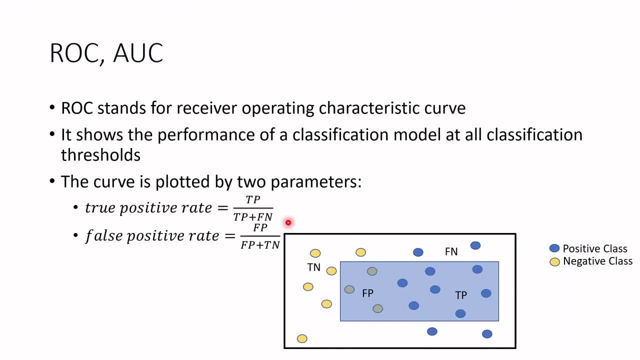 rate to be well as low as possible, because what we want to have more true positives, and we would like to have a well less false positives, and if you search for an ROC curve online, you'd probably see something like this: what we have over here on the horizontal x-axis is the false positive rate, and on the y 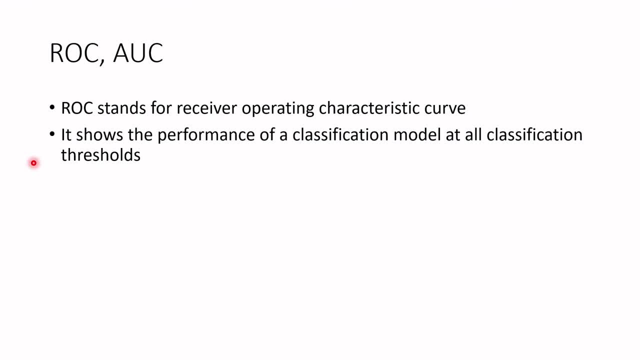 we calculate for many thresholds. well, that's what we do over here, is that we calculate for a given model and for each threshold we calculate two different parameters. The first parameter is the true positive rate and if you remember from the previous slides- 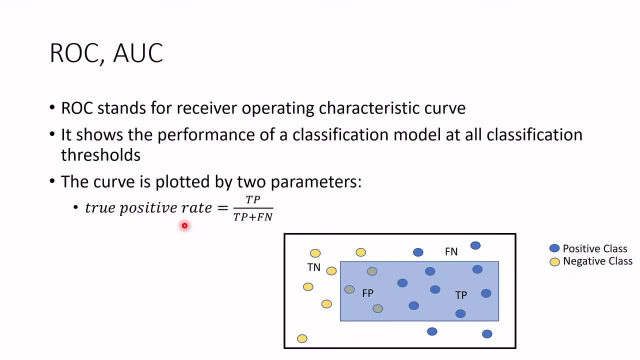 it's the exact same thing as recall and sensitivity. It's true positive divided by true positives and the false negative. So how well did your model perform? regarding the positive class, The next parameter is the false negative. The next parameter is the false positive rate. 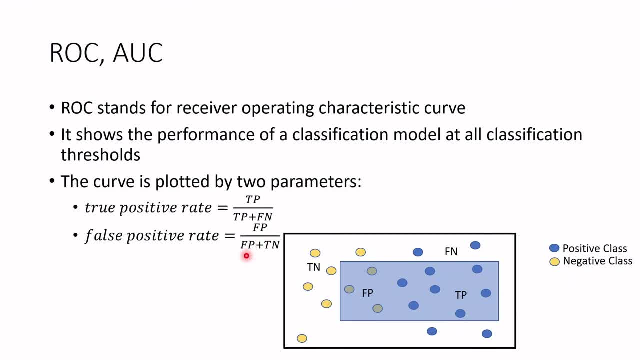 which is false positive, divided by false positive and the true negative. So, putting that into words, it's out of the negative class. in how many instances was your model incorrect about? And intuitively, we want the true positive rate to be as high as possible. 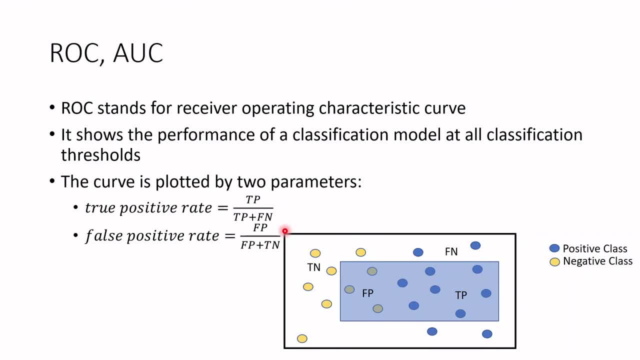 and the false positive rate to be well as low as possible, Because, well, we want to have more true positives and we would like to have well, well less false positives. And if you search for an ROC curve online: 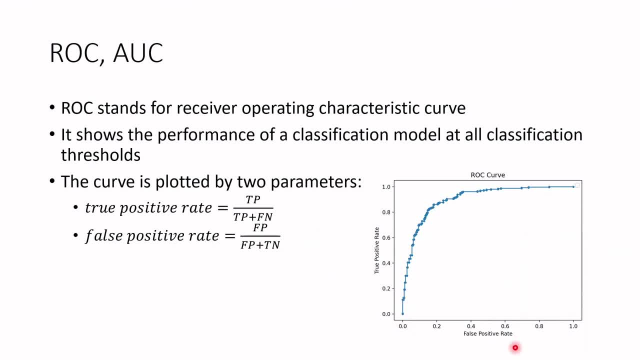 you'd probably see something like this: What we have over here on the horizontal x-axis is the false positive rate, and on the y-vertical axis we have the true positive rate. So the best threshold performance would be at this point over here. 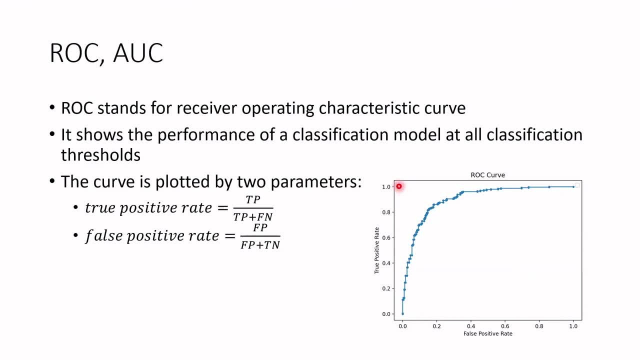 one for the true positive rate and zero for the false positive rate. Obviously, that's very hard to achieve, And well, what we have over here is a different dot. Each dot represents a different threshold, and well, that helps us choose the best thresholds. 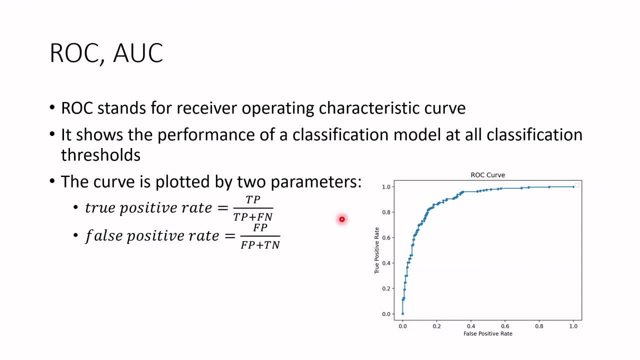 that we would like to use for the model. That's one use: choosing the best threshold. Another use is when you compare different models, and that's where AUC comes into the picture. AUC stands for area under the well ROC curve. 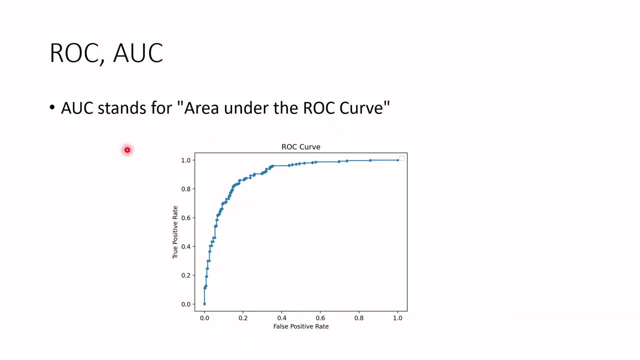 And well, if we have two different models and for each model we have an ROC curve, the first model would be represented by the blue ROC curve and then, well, the next, the second model, would be represented by, let's say this, red curve.